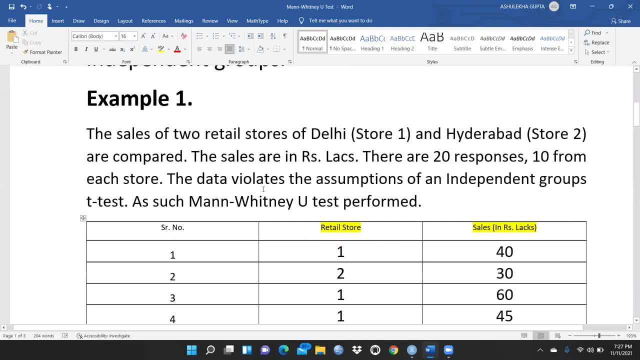 the sale of two little stores of Delhi. let's say we had given store 1, right. store 1, Delhi and Hyderabad is store 2 are compared, The sales are in rupees lakhs and there are total 20 responses. we had collected 10 from each store right and the data violates the assumption of an. 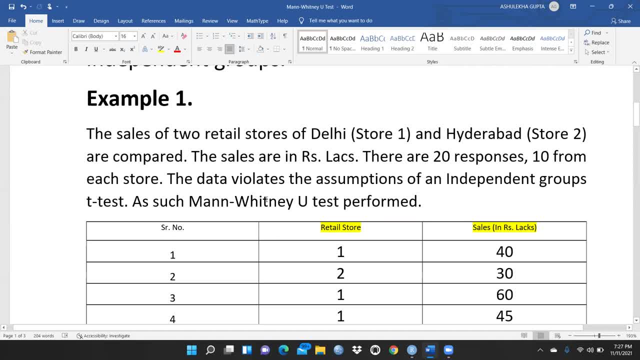 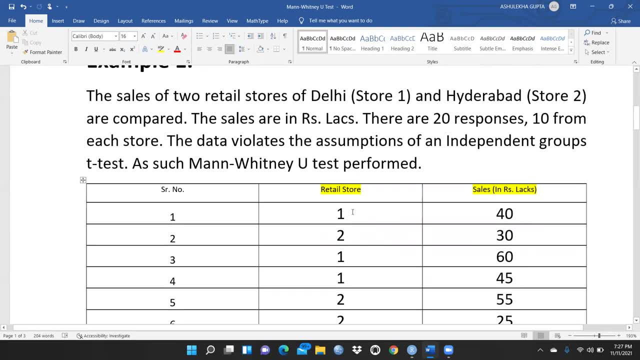 independent groups t-test as such, Mann-Whitney u-test performed. So what happened? Because this data is not normally distributed and there are two categories, we have taken two retail stores, one that is located in the Delhi and one is located in Hyderabad, and one 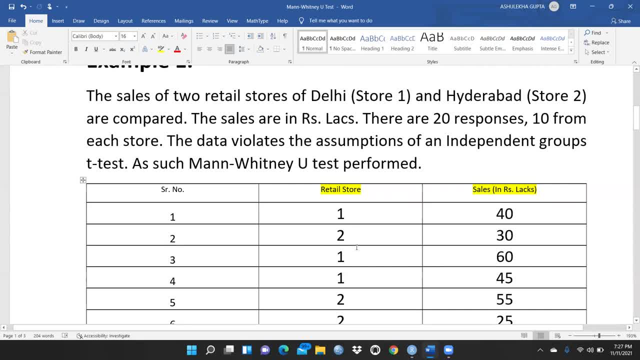 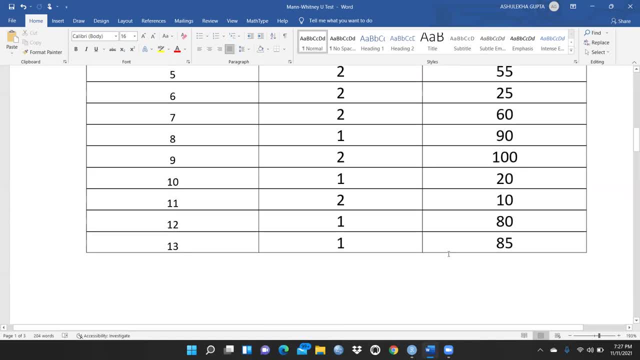 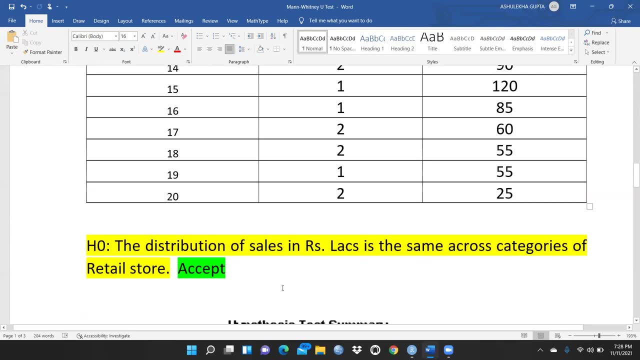 coding we had given to Delhi and two we had given to Hyderabad, and on the right hand side you can see sales sales that is in rupees lakhs. So what is our hypothesis? Our hypothesis you can see here: the distribution of sales in rupees lakhs is the same across categories of retail store. 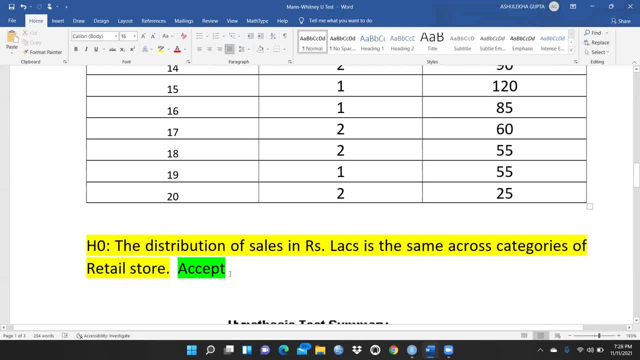 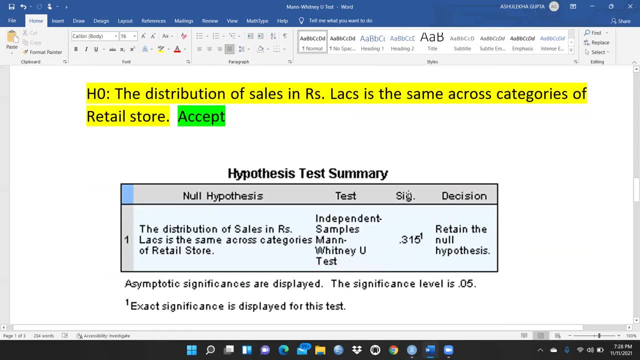 So when I had applied SPSS, it was accepted. I will give you this link in my description box: that was accepted So you can see this was the result through SPSS and through SPSS, the, on the same data I have run, and you retain the null hypothesis. that means we will fail to reject null hypothesis at the. 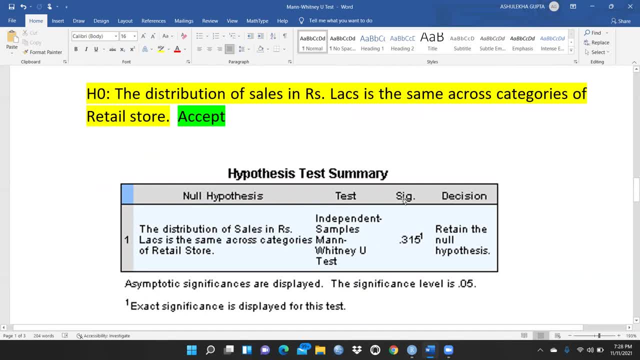 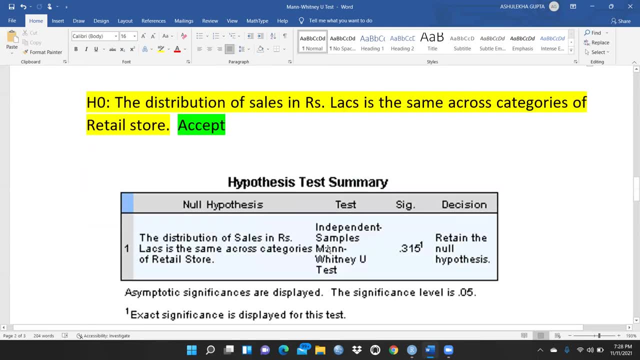 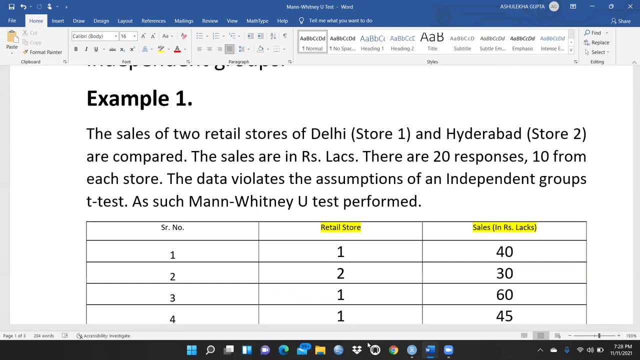 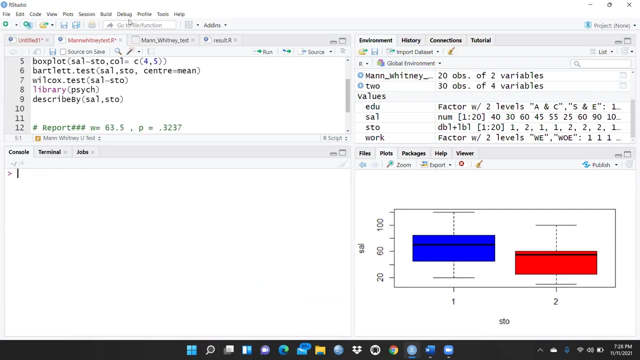 significance level 0.05. that was the result we have got now. these were the t statistics, right, wilcox and jw and all. so now what we have to do now the same data we would like to test in r and how we have to run. fine, let me first clean all these things. i am just cleaning. 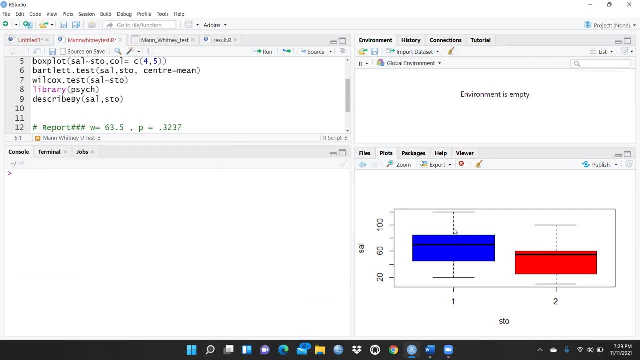 all these imported values and this plot also. i am cleaning right now what we have to do and this file also. man by tv are closing and you can see here i am. i just closing this. this is the. this is our, the script file. so, first of all, 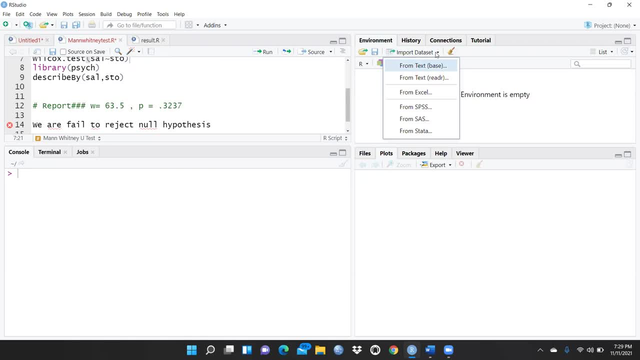 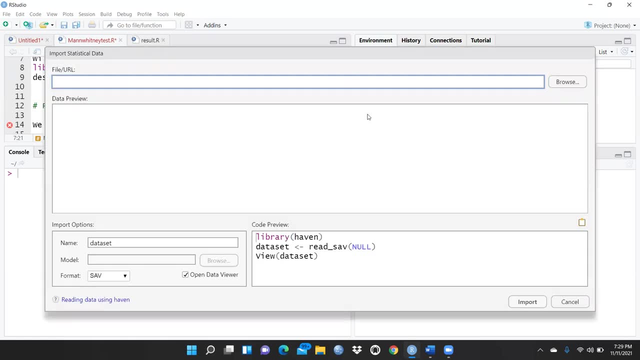 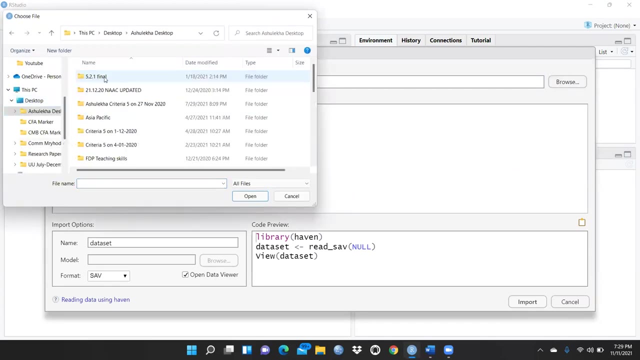 all what I will do. I will import my data set. I will import my data set because this is the SPSS file I had already run, so I will use the same file, SPSS file, where this file is put it here. so let me check. that is on the desktop and it's still. that is put it in my R folder and R studio folder. 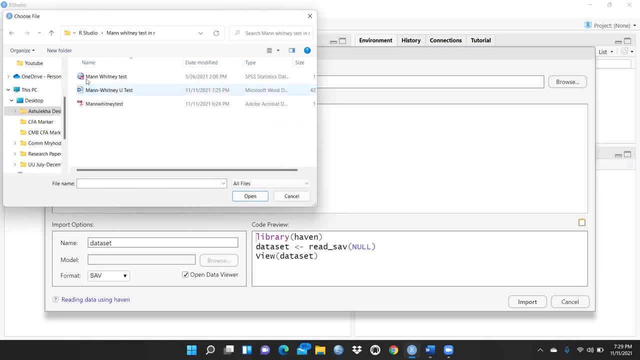 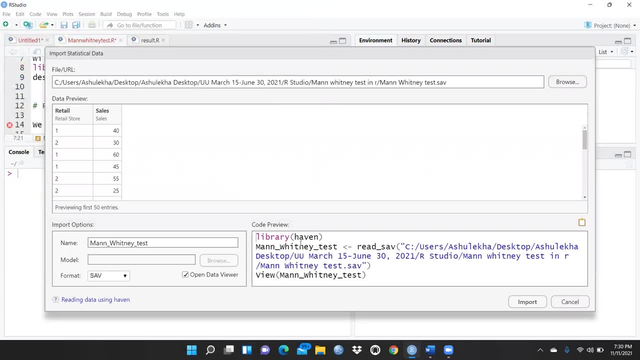 and in the R studio folder you can see man wait me and you I will use this SPSS file. I will open this file and you can see this one is the library heaven that is required to open any if first time you are using, first time you are opening this SPSS file. so you must install this library library. 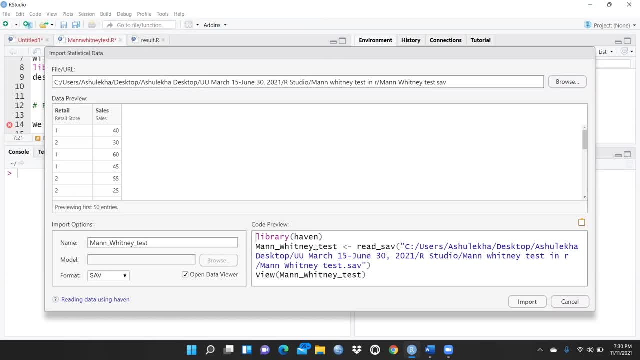 heaven is required because I had already used in my R software number of times SPSS file, so I had first time when I used, so I had already installed this SPSS file, so I had already installed this library hub that I will import. so now you can see this file is open retail. there are two columns. 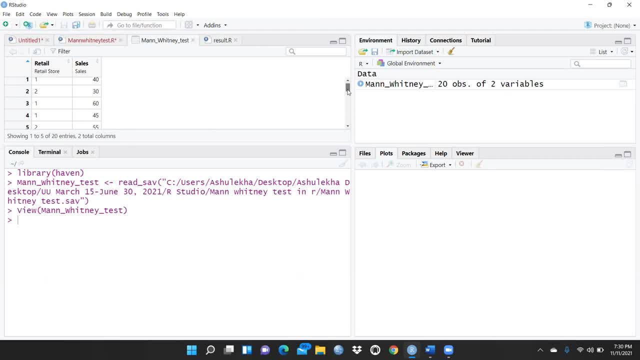 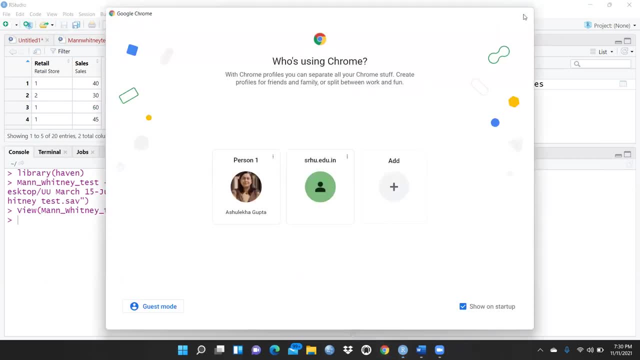 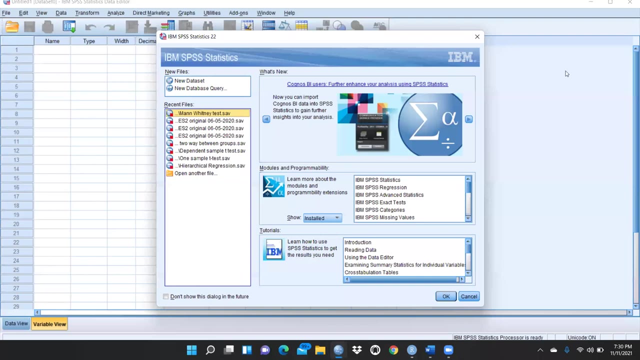 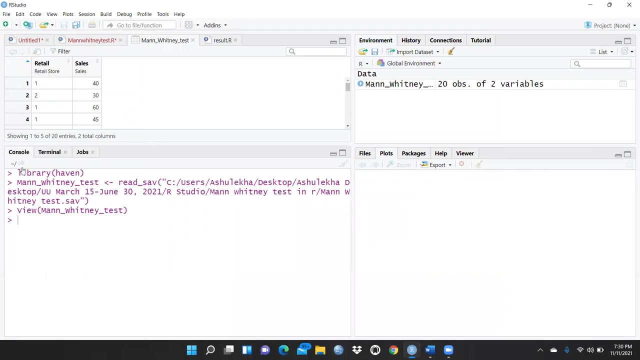 same file, retail and sales, and I will show you this file also how I have done coding like SPSS itself. right, you can see this file is, I think that is not open- one we had given to Delhi and two we had given to Hyderabad city. so now what we have to do. first, I would 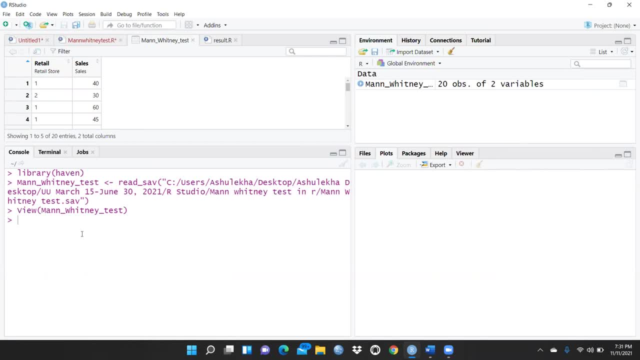 because this one is the very long name, manvaitni test. so simply I am putting up one name. I will. I will write here right. this is my one variable. I am creating where I will put this file- manvaitni test- right? so i will press enter. you can see in the environment: uh, man, white knee. that was the file. 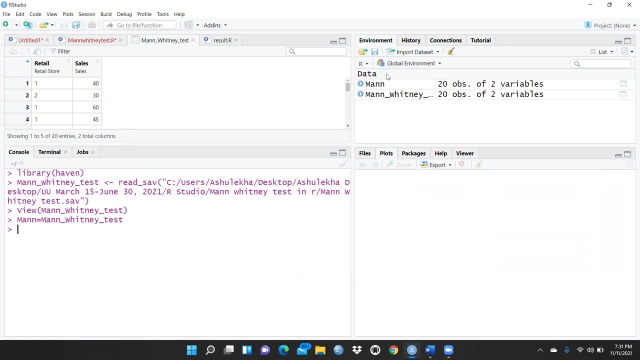 is open: 20 observations of two variables. that name is very long so i had put it, this file in this variable. now, what i have to do, before running any test, let me create, because again and again i will not try dollar sign right. so what i have to do, let me create. uh, one, i'm just writing. 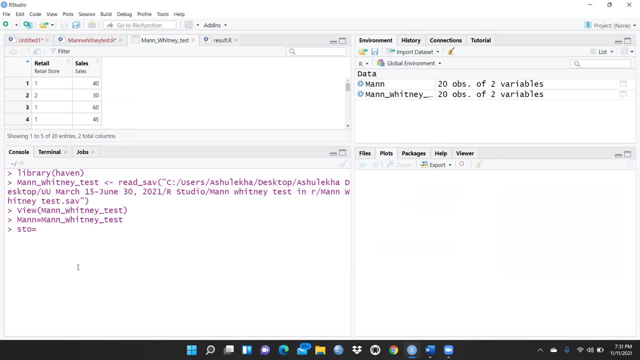 this store, this white variable i'm creating over here and from where it will pick up. this one is the man, is the one variable i had already created, dollar sign and this retail. that means this value i am storing in this variable. so what is happening? and let me try to take one second, i will not try dollar sign. i will not try dollar sign. 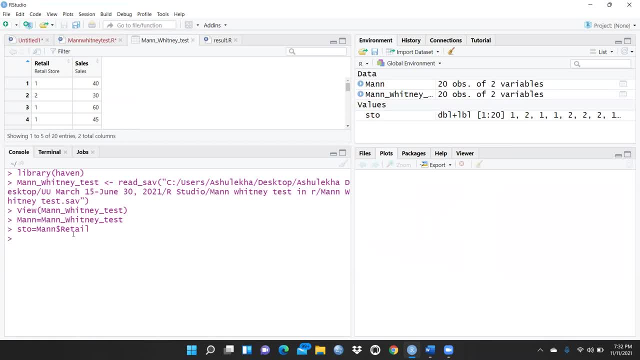 you can see here, this variable is created here and these values retail store values are. i had put it in this variable, so, rather than i will again and again, i will use this one is the long man and dollar sign and this retail. simply, i will use sto and same thing i will do, i will perform. 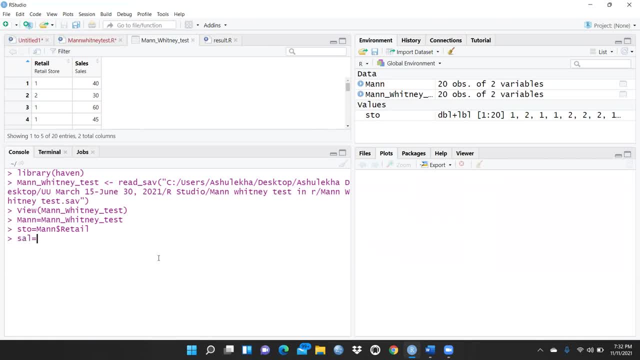 with sal cell sales. and where is this sales variable? in this same file. and again i will press dollar sign and this sales variable i will put it in this variable. so now you can see here both the variables are here, and uh, script how you have to write. i will tell you. here is the file. 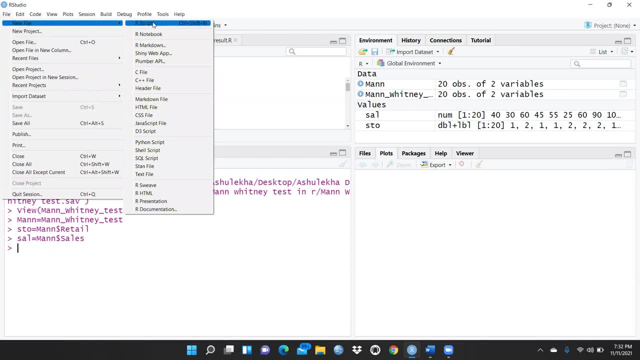 when you have to press new file, our script, so new window will open up and here is you can write the version of the trial. so i will tell you how to write the script. and here is the script. and here is the file of 2018 and this is the file of 2020 and here is the version of sampai. 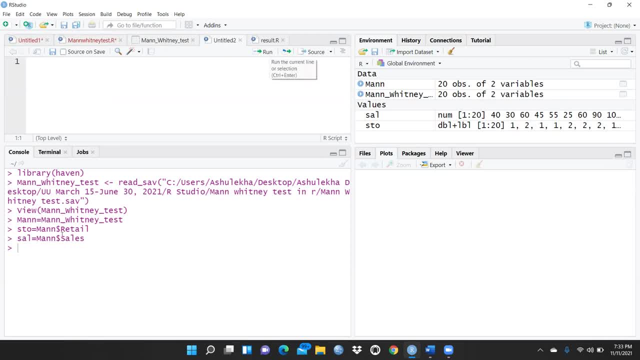 write your script and after that, simply you can run. so before I mean, rather than you are writing directly in console, you can first write here or you can run and these come, these codes would be reflecting over here. so what I have to do, I had already let me close this file. I don't want this. 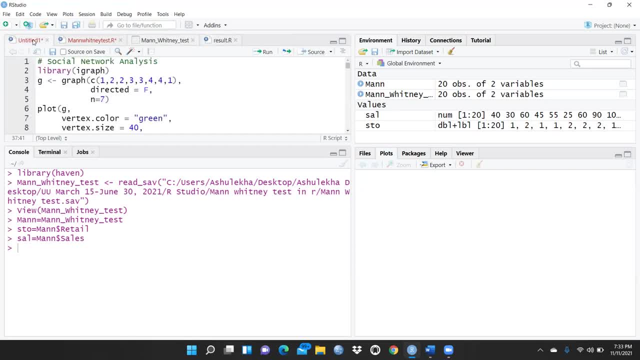 file because I had already created some script. yes, here is, I had already created, because a moment you will press here right, you will click here run. first of all, we want to check box plot, right? so rather than I am writing here box plot, you can see here. fine, either you can run from this. 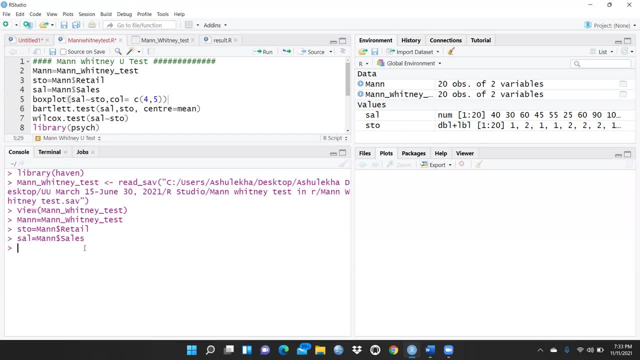 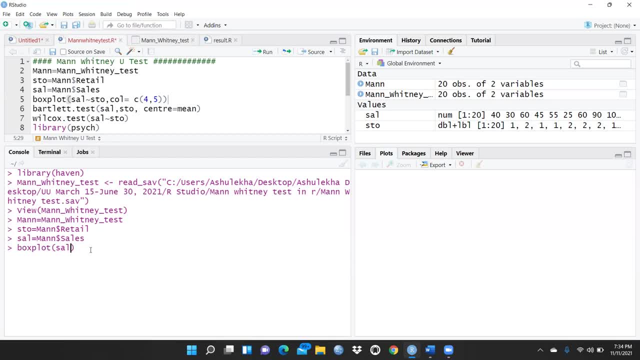 simply, I will use box plot. in between, I will use this sign and after that I will use this toe and I will write color, what color combination I require. so simply, I want to use these colors. right, I want to use color. let's say, I am using inverted. 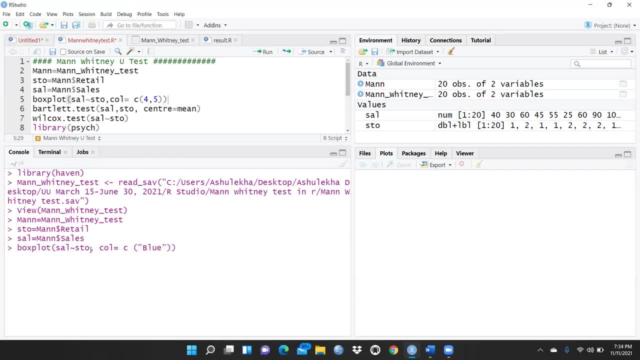 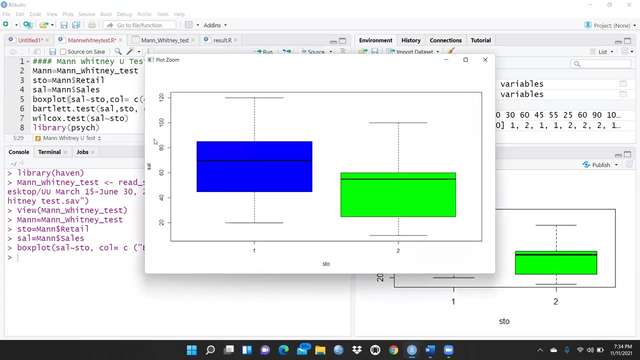 commas and I will use blue color and I want to use, let's say, one more color, that would be green color. so simply I would write, or otherwise you can write, or color code also: four comma five, so that would also be give you similar results. so you can see here I will zoom this- both these box plots are here. 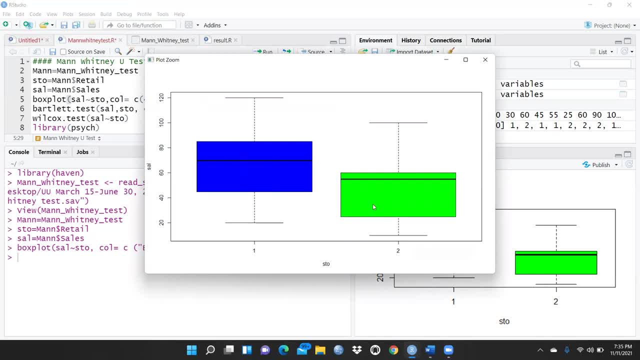 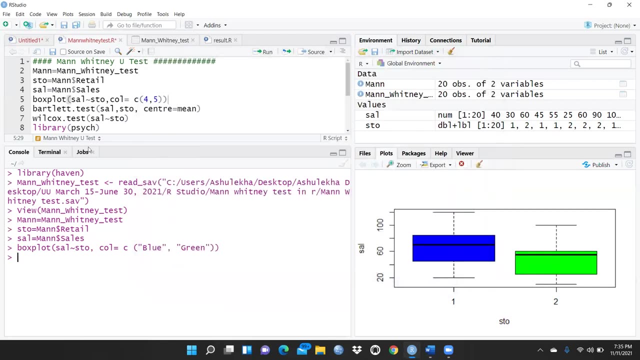 this one is the because first box plot I had given blue color, another one I had given green color. the same colors. it is reflecting here and it is reflecting this. the mean value of both these box plots and my data is now what I have to do after this. I will give you the same color, color. 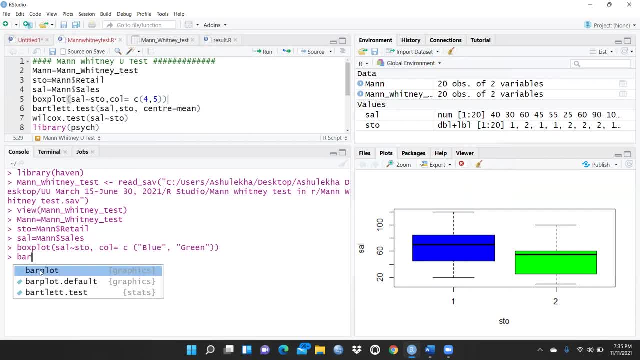 I would like to check homogeneity test also, so I would use this. this one is the mar décidé test and what I have to do, sal, this is my one of the variable and store and I would use right, center equal to mean. center equal to mean. 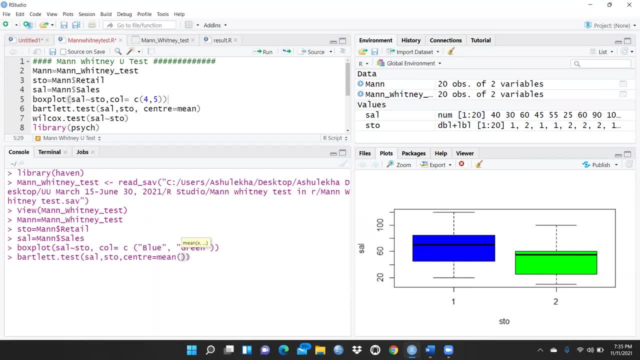 correct and I would center equal to mean, simply mean I think I don't require this thing. then I would press enter so you can see p-value is 0.9742. so that means our data is. the homogeneity is here right in between both these variables, because p-value is greater than 0.05. now what? 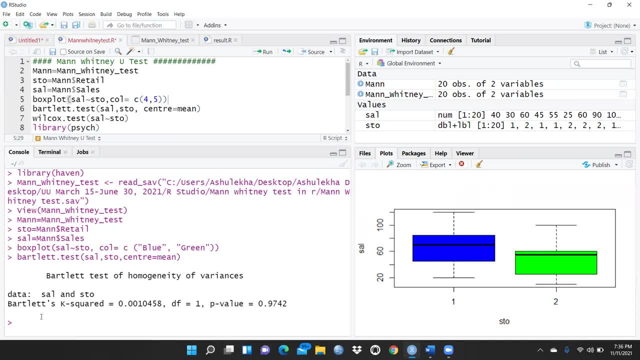 I have to do. I would like to run Mann-Whitney test. so Mann-Whitney test is as you have seen in my statistics. also, there is the one test you will type here: Wilcox, right, Wilcox test. if it would be functional, it would be automatically, will be reflecting over here and this test in. 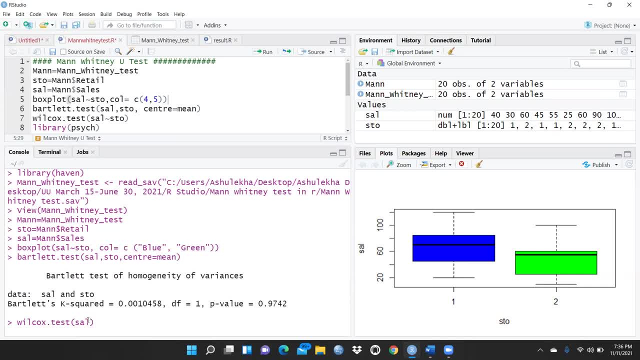 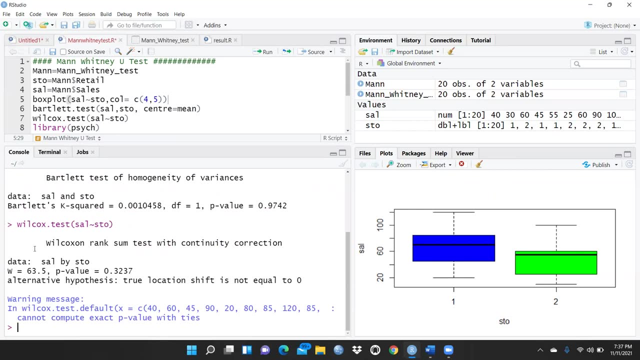 between my sales and across the cities. you so sale and stores and then I would press enter okay, so now you can see these are the results reflecting over here, right w value of w. you can copy this test also and you can report in your research paper or you are writing any thesis. 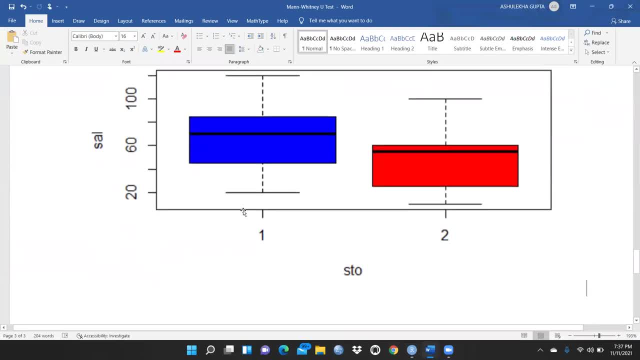 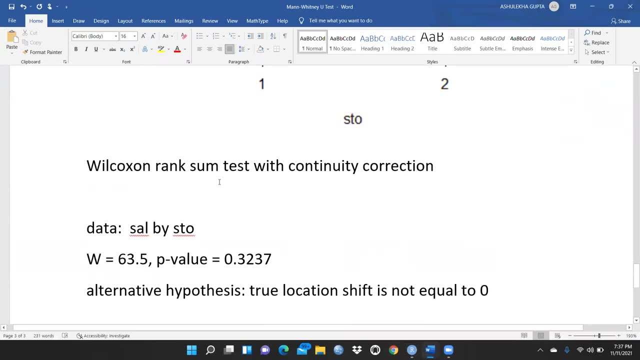 and all so you can report here. this is my SPSS results and this box plot I had already copied here and I would press enter and then I would press enter, and then I would press enter and then I will tell you how you have to copy. and Wilcox, and rank some test with continuity correction. 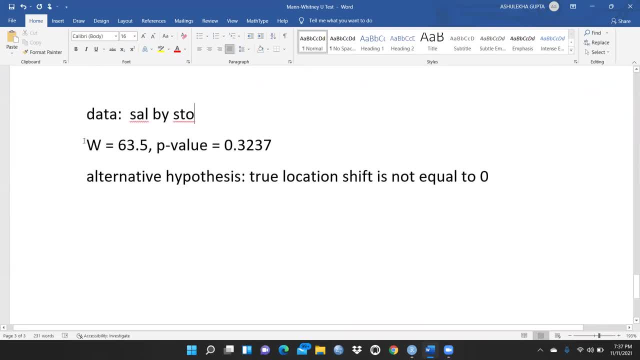 right and there is the. you can see w value of the w is 63.5 and p-value is 0.3237. it means an alternative hypothesis: true location shift is not equal to zero. so that means when the p-value is greater than 0.5. so what we have to do- the through r also we have to do- is we have to do the p-value. 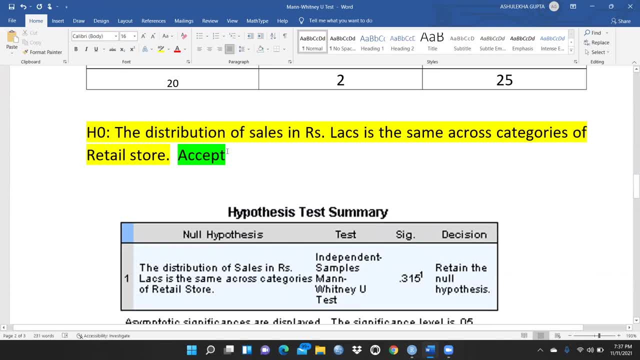 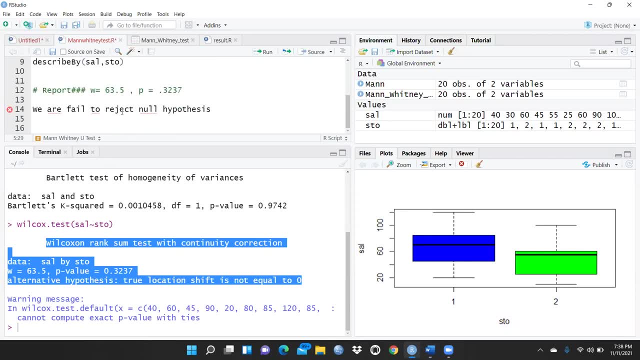 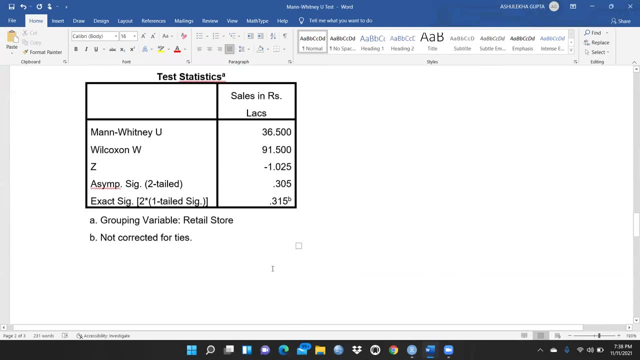 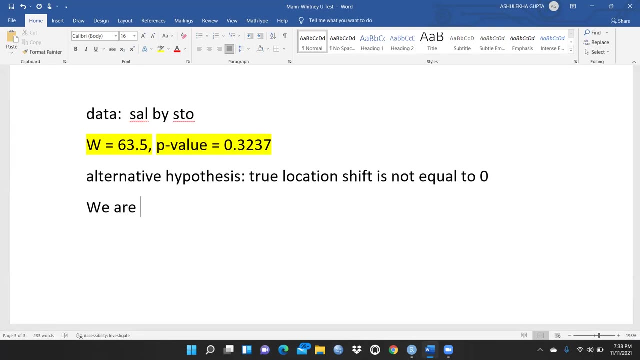 so this null hypothesis is accepted, or we can write here how we have to report our this results, so we can write here. I had written here: we are failed to reject null hypothesis, so you can write: we are after this. you will write how you have to report. we are failed to reject. 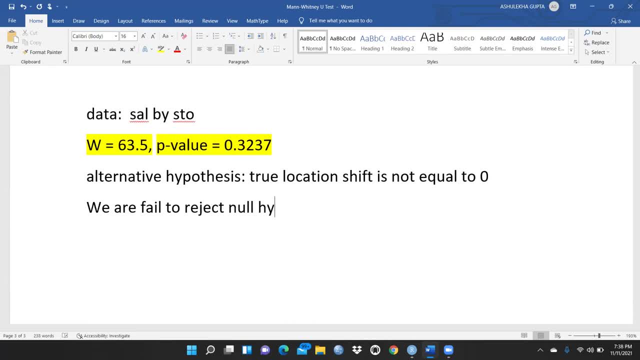 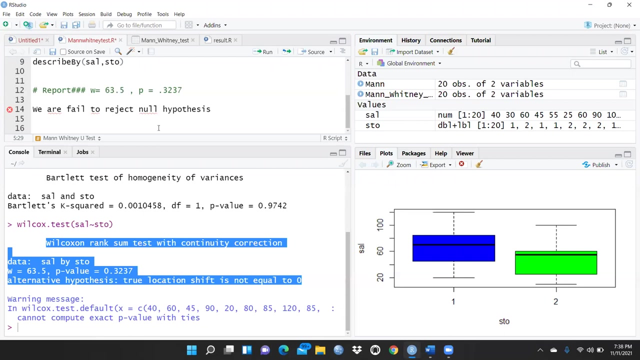 null hypothesis. null hypothesis, right. so I'm sure, through both the ways what happened? same results we are getting, whether we are running through SPSS or the same test we are doing in R. so that means same results we are getting. but after that suppose you want to know mean median, high value, Etc, so what you can do. 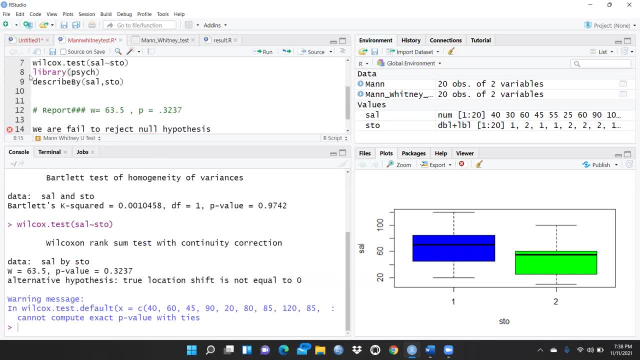 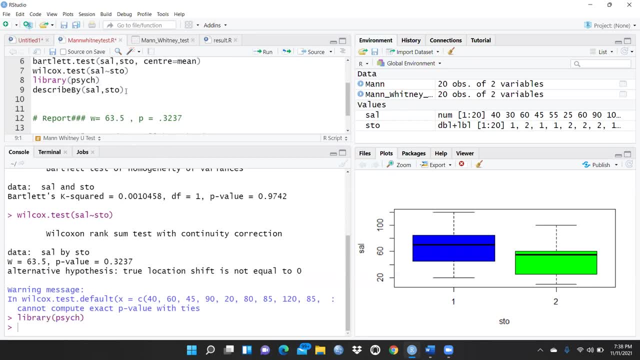 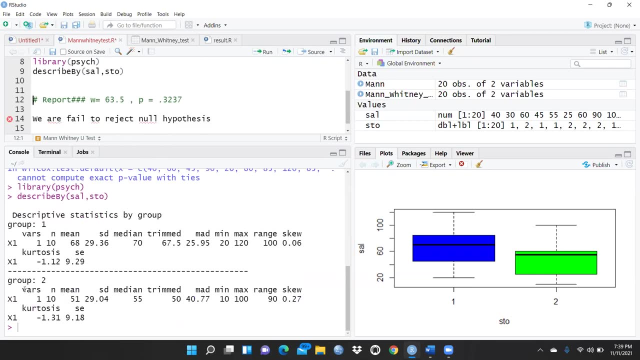 you can simply install a library psyche, so here is library. then you have to press this, run right, I had already installed, and after that you can use this, what is described by, and both these variables you have to write, and you can see here descriptive statistics by group, because group one in my first group data is from: 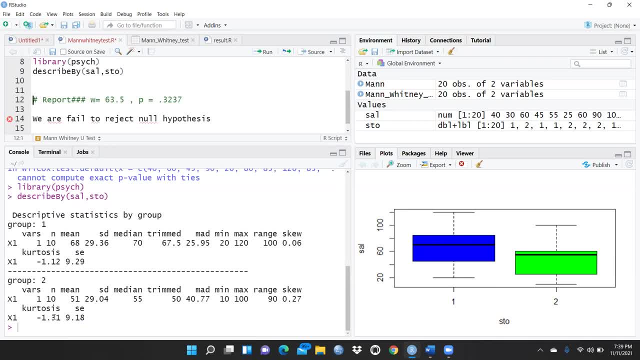 Delhi. right, there's the one city, Delhi. another city I have taken to second city. I have taken Hyderabad, just comparing whether there is any difference in the sales right. so i had it. through this man whitney test i had already proven we have failed to reject null hypothesis. that means there is no. 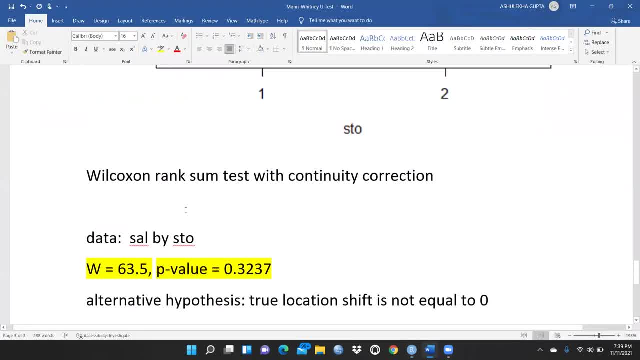 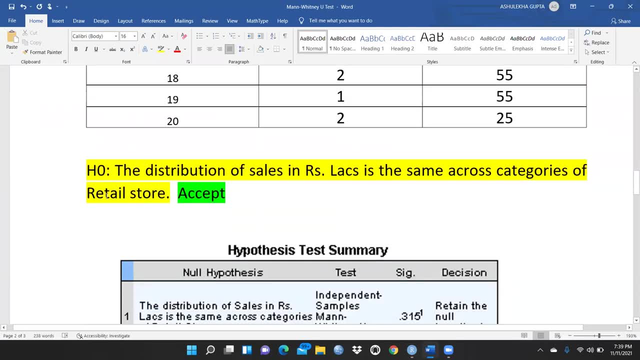 difference between these two. i had already said here, written here, the distribution of sales in rupees lex is the same across categories of the retail store. that means both these cities are these. this is where the sales is same. so what we have to write here now you can see here. so this: 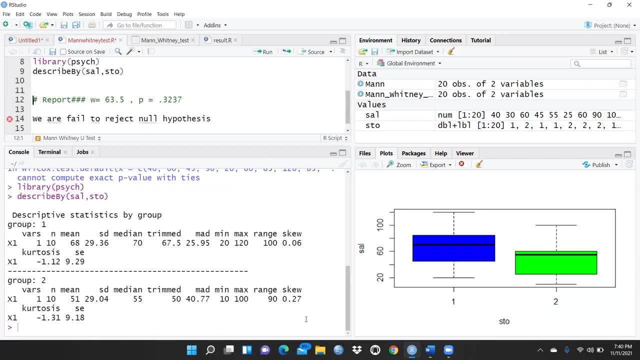 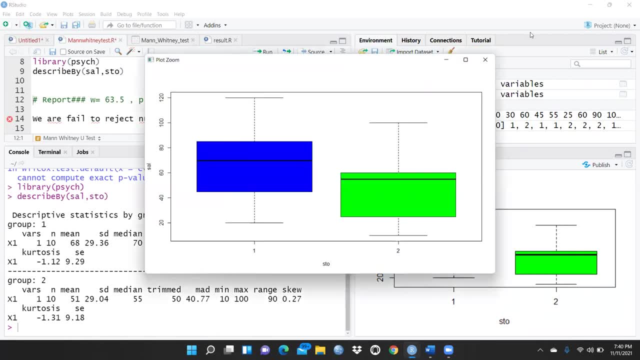 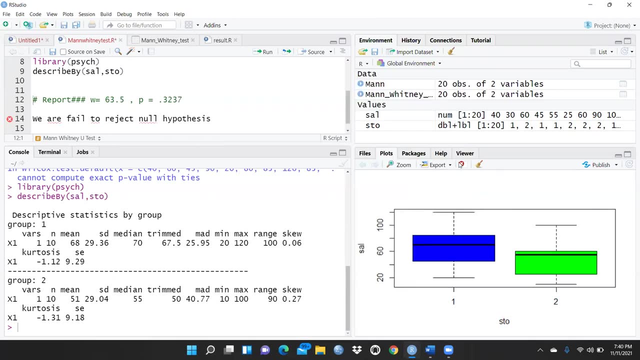 one is a descriptive statistics also. you can copy from this place and you can report there now how you have to copy this plot. you can zoom this. you can see here right and after that what you can do: export, copy to clipboard. i mean other ways also. let me explain you other ways also this: 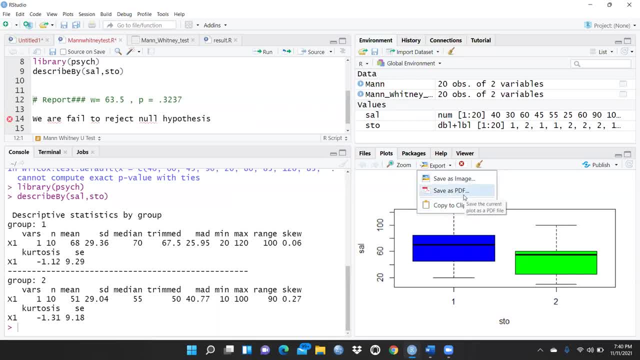 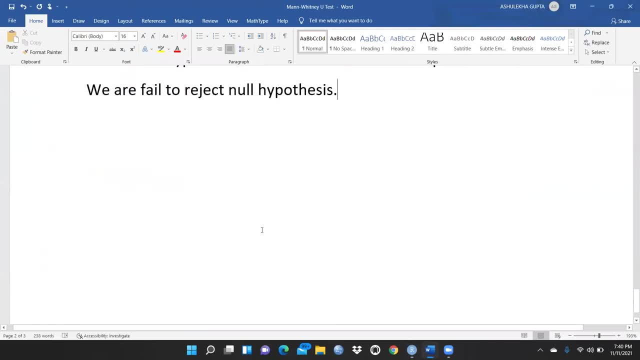 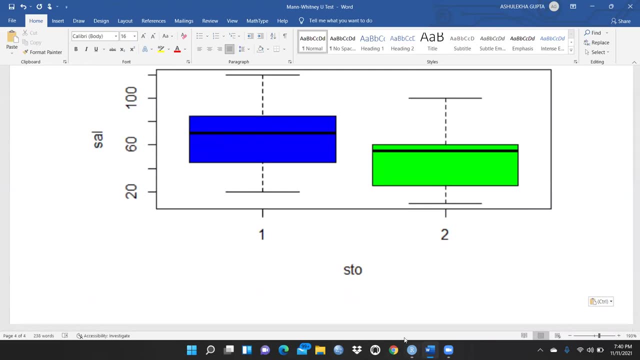 is the. this is the. this is the. save as image, save as pdf right and copy to clipboard. so i'm just copying this clipboard and i will put simply this box plot over here. simply i will press this ctrl v and both these box plots you can report in your research paper. one more thing: suppose you want to know about this. 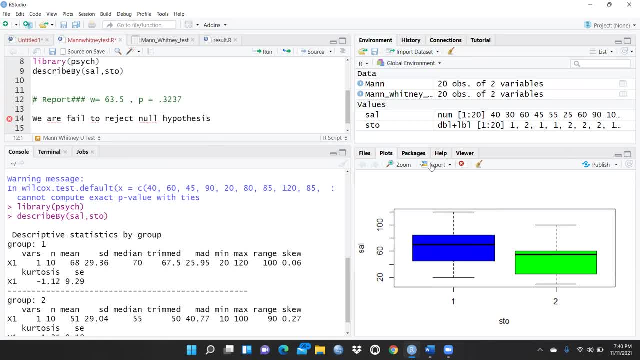 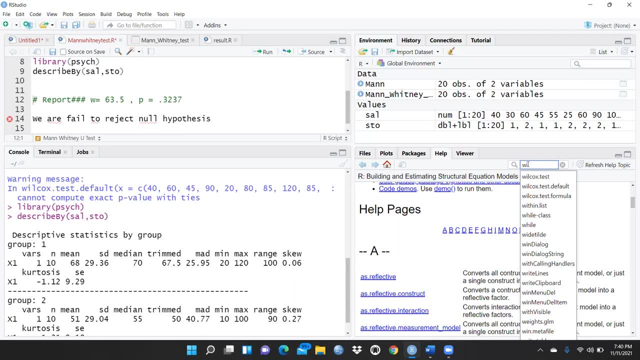 what is this test, wilcoxtest? so simply, you have to go to help. you can write, because this is the beauty of the r, everything is written there and what you can do, you can simply type here, right automatically it will come and you can press and everything. description is here, you can see.